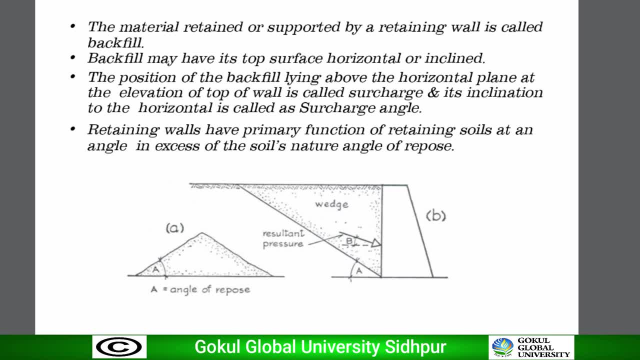 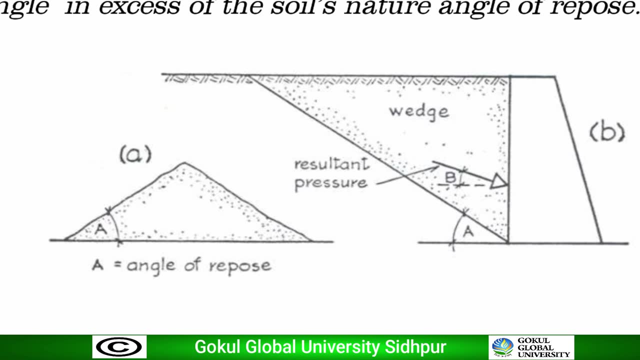 and the retaining wall have preliminary function of retaining soil at an angle in axis of the matri soil, natural angle of repose. so here the present a is the angle of repose, the arrow show the resultant pressure and the triangular look like wedge, soil wedge. this is the 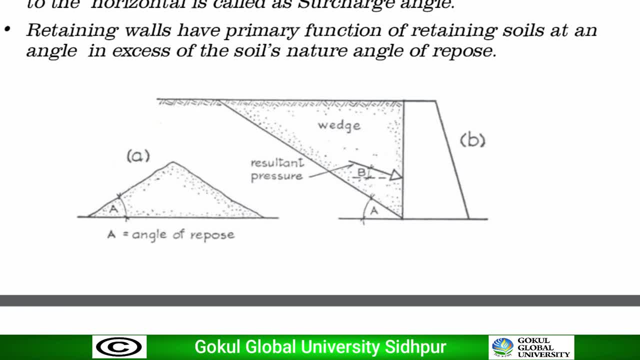 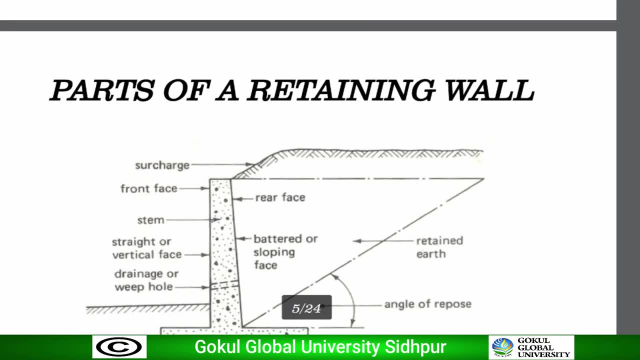 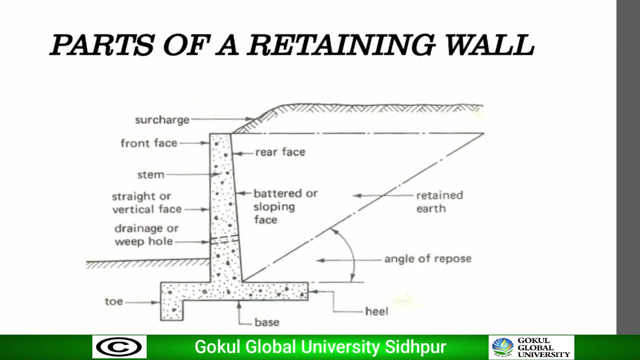 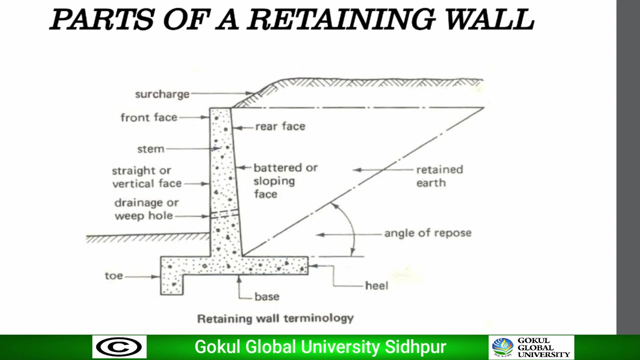 part of soil, earth pressure. now we are discussing about part of retaining wall. the first one is surcharge. surcharge is the load that are on retaining wall. these are the front side stem. there are main component of retaining wall are. there are five main component of retaining wall. first one is stem. here 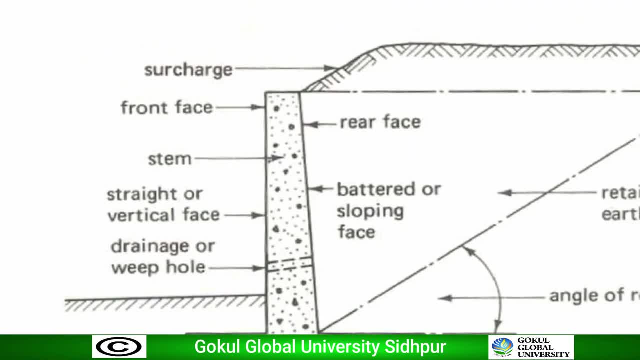 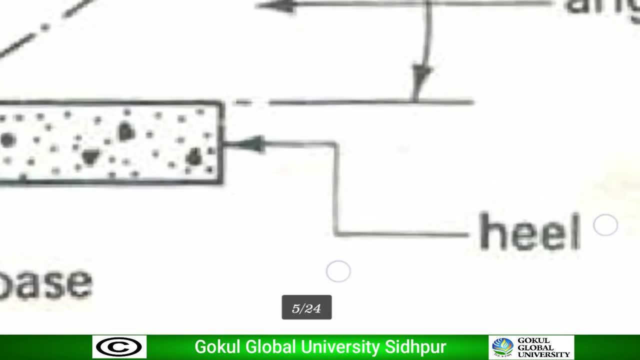 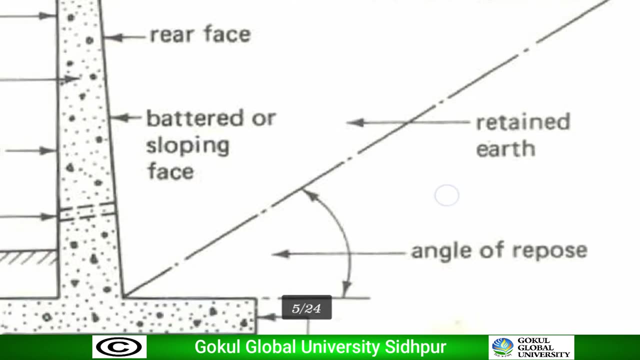 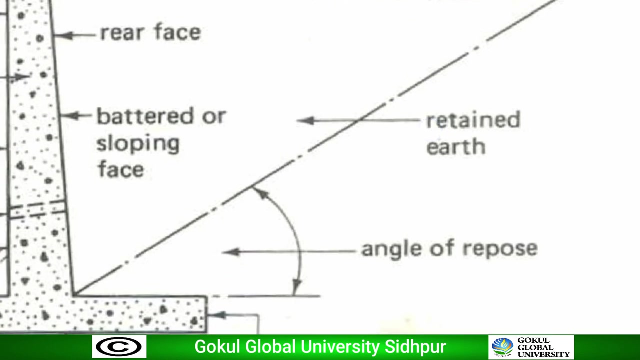 stem. stem is shown. second, one is toe slab. this one is toe slab. third one is heel slab. this one is heel slab. fourth one is counter fold, the arrow, the retaining earth. this one, this dotted line, are shown as counter fold. counter fold in case of counter fold, retaining wall. 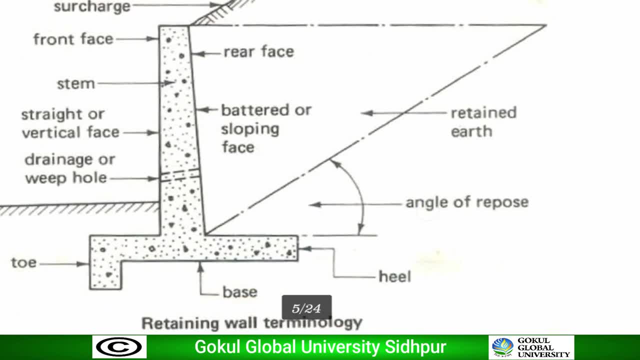 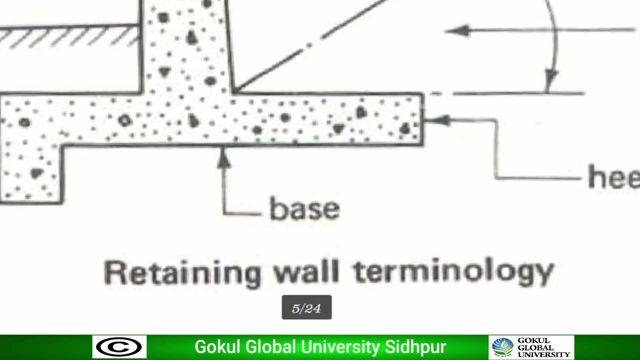 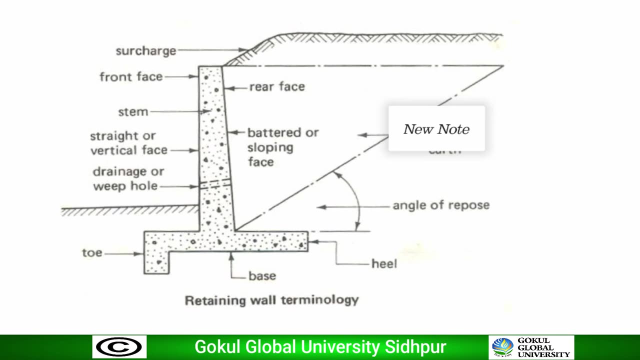 only ok, full name. a is shame key and this one is shear key. from the base of tuh retaining wall terminology. ok and uh. and the important question is where the application of retaining wall first one. where the retaining wall is used first one to avoid the pit stop, duct the rock. 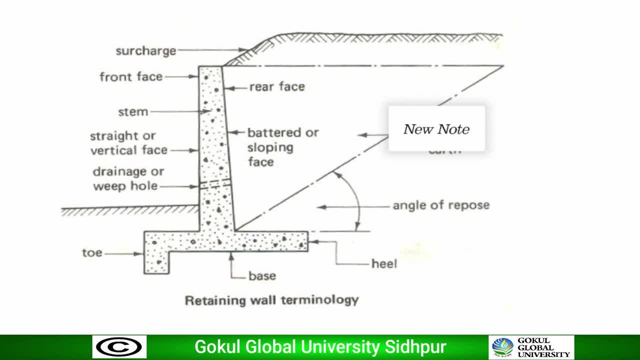 tilling area. second one: a slide wall of bridge approach side. third one to provide lateral support for embankment. fourth, one constructed porthole, the jetden, and the other one is hitting surface in solid- is here here. this is the path of the retaining wall. then these are the two. 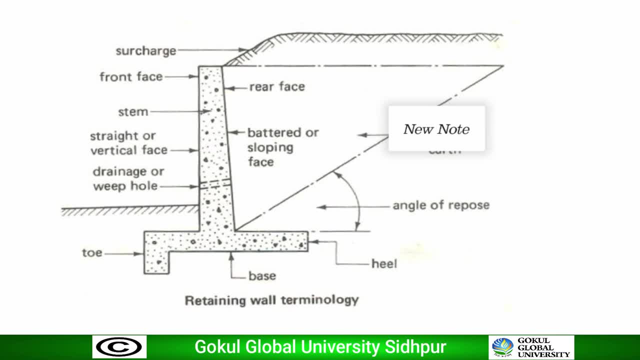 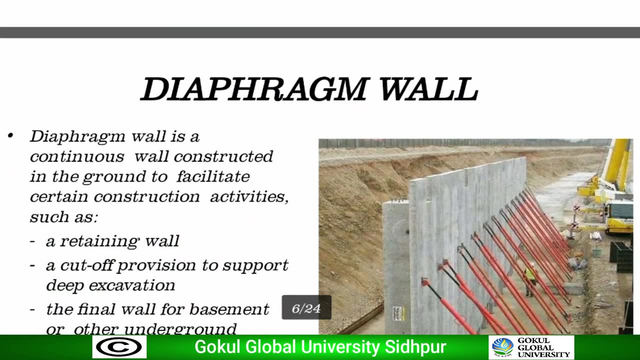 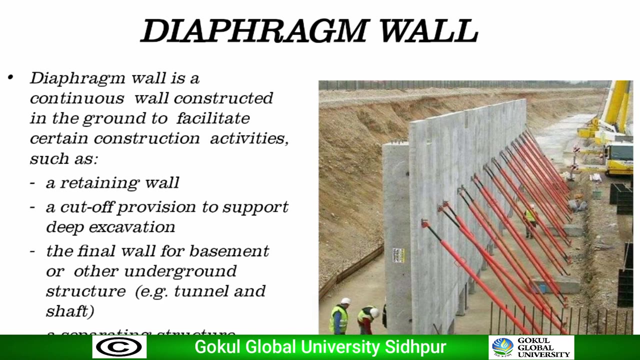 construction of basement below ground level in building. so these are the different application of retaining wall. now we are discussing about diaphragm wall. what is diaphragm wall? a wall construct constructed in situ by special trenching method to act as cutoff wall or serve as a structural member is called a diaphragm wall. the standard 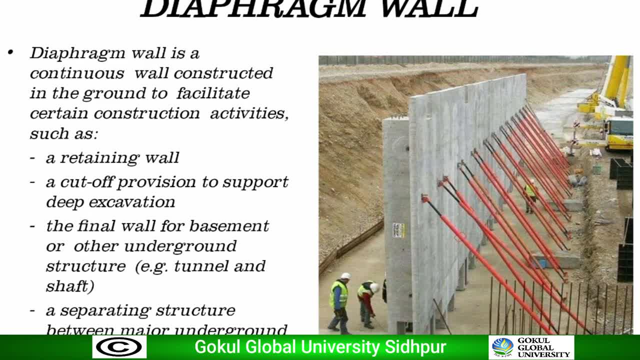 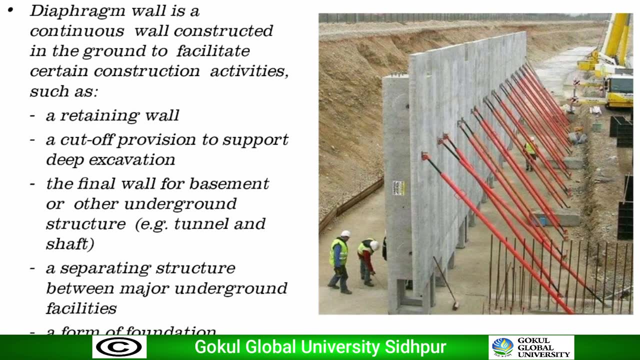 width are 100 to 200 mm for cutoff wall and 450 to 450 to 1000 mm for structural member. okay, in figure we can see the diaphragm wall. the diaphragm wall are pre-constructed, pre-constructed, pre-constructed type retaining wall. 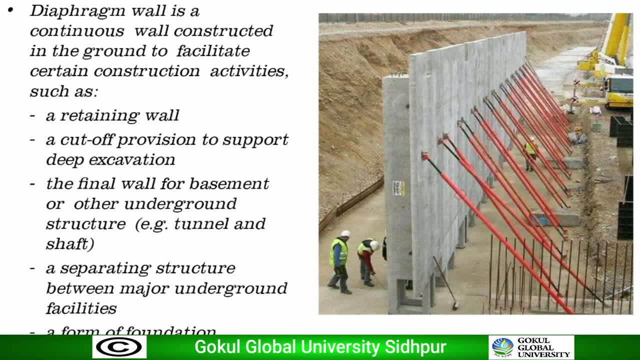 diaphragm wall is a continuous wall constructed to ground to retain construction activities, such as retaining wall, cutoff provision to support deep excavation, as the final wall of basement or other underground structure, as a separating structure between measure underground facilities, as a form of foundation. okay, diaphragm wall is a reinforced concrete structure. 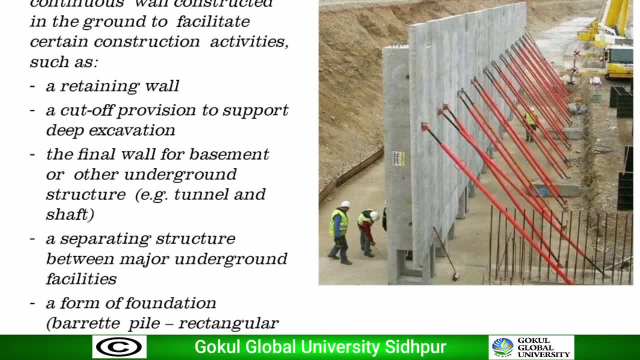 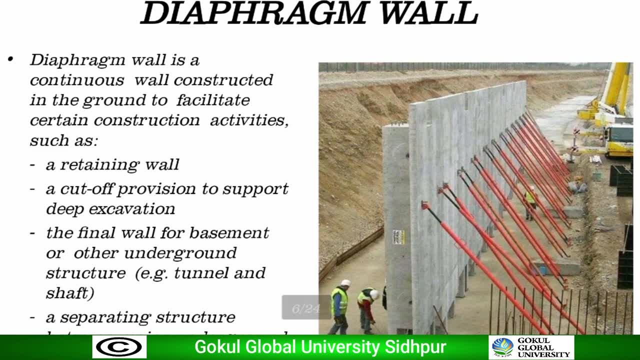 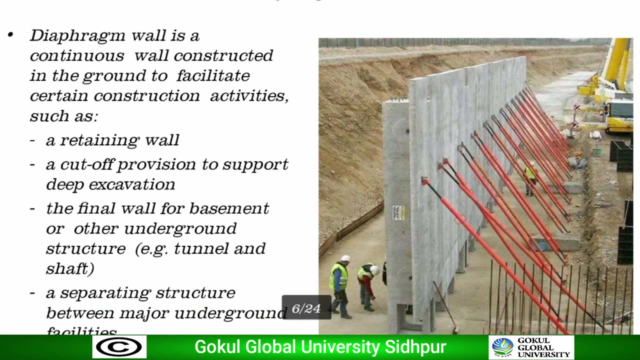 constructed in situ panel by panel. the wall is usually designated to reach very great depth. just remember that diaphragm wall is used to reach very great depth times, up to 50 meter. mechanical excavating method is does employ. okay, in figure we can see that diaphragm wall is a reinforced concrete structure constructed in situ panel by panel. this one panel. 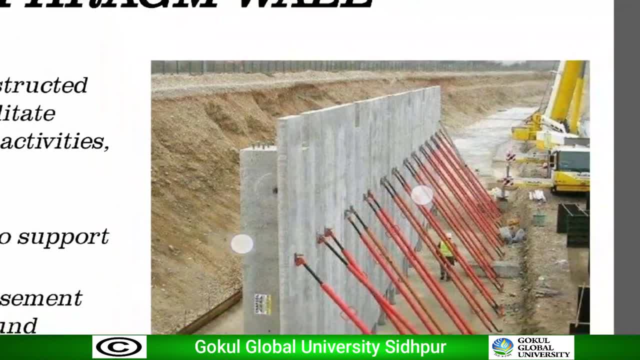 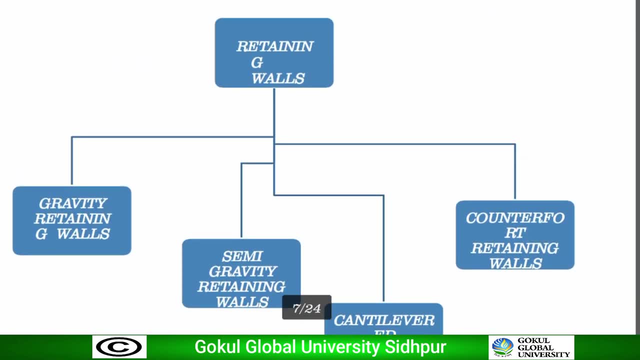 by panel. we can see that in the figure. okay, these are the part of written. these are the different retaining wall. first, one: retaining wall written. there are the different types of retaining wall. first one: gravity retaining wall. second, one: semi semi gravity retaining wall. third, one: can deliver. 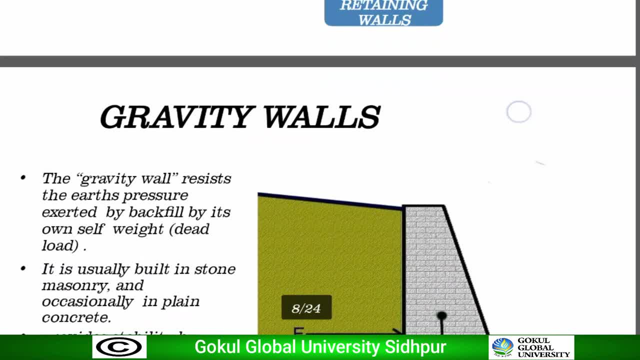 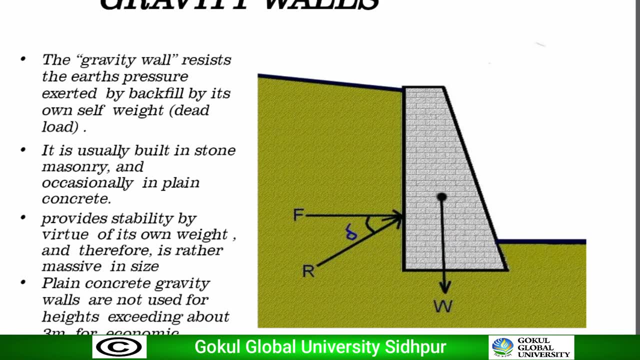 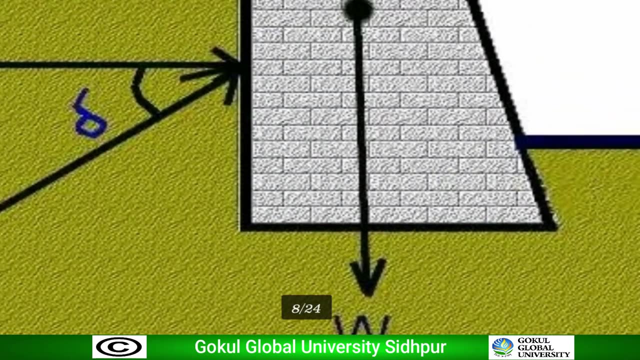 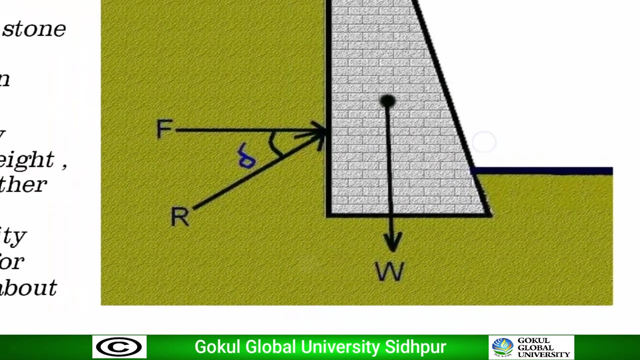 retaining wall. and fourth one is counter for retaining wall. so first one gravity retaining wall. gravity retaining wall is made of plain concrete or brick masonry. the stability of the wall is maintained by its own weight, maintained by in in what, in its own weight, it's called a W. it's one way. it generally made up to height of three meter of. 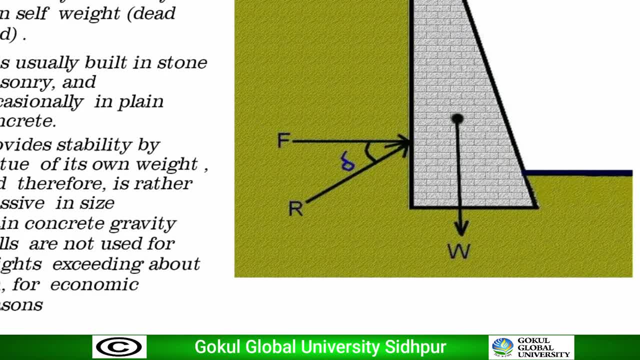 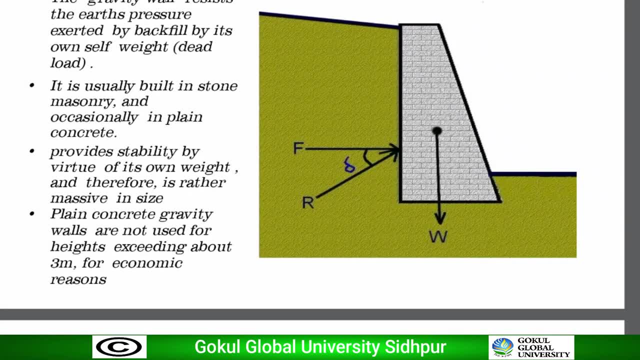 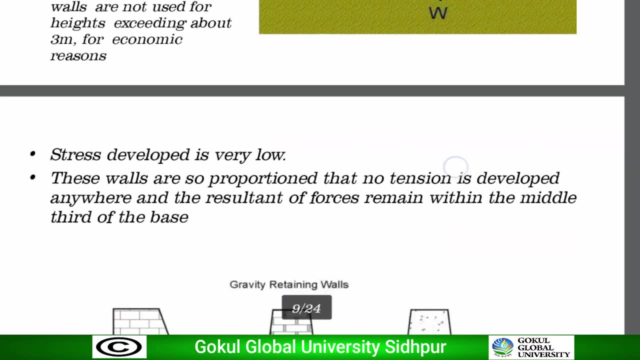 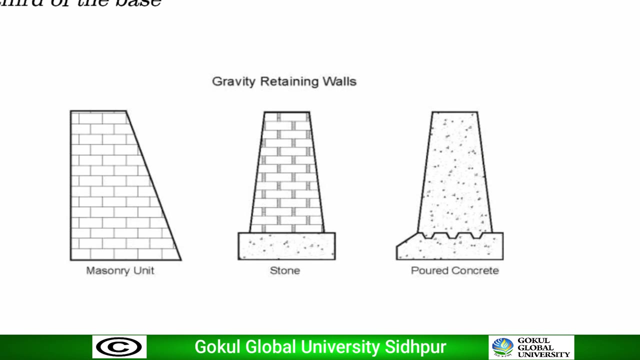 wall. generally, where the height of this is a height, the requirement of height is three meter- wall gravity retaining wall is constructed. remember that R is a resulting. R is the resultant force acting on the retaining wall. okay, gravity. we can say that the gravity retaining wall is made up of plain concrete, masonry unit or stone types. we can see that in the figure: gravity wall. 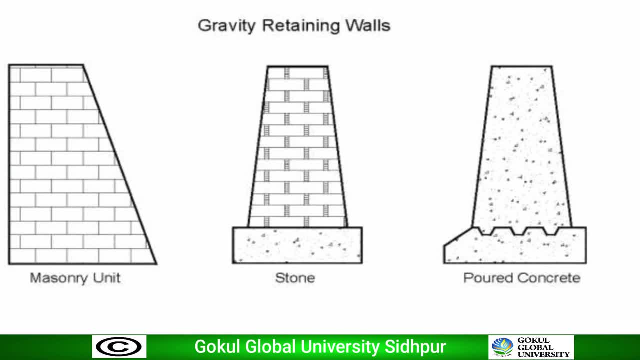 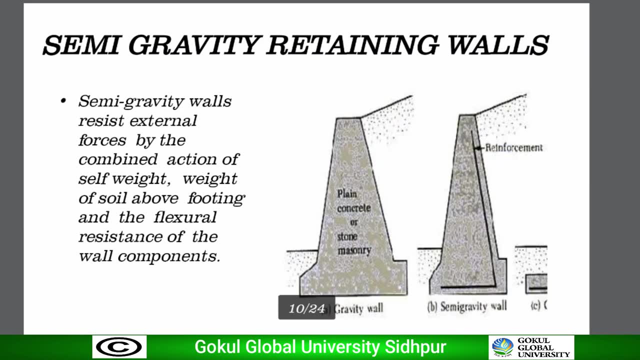 retaining wall masonry unit. second one is stone unit and third one is Paul Paul concrete. second one is semi gravity retaining wall. semi gravity retaining wall resist external forces by the combination action of self weight, weight of soil above footing and the flexular resistance of the wall component like stow stem, slab, shear key. these are the member that resist the external. 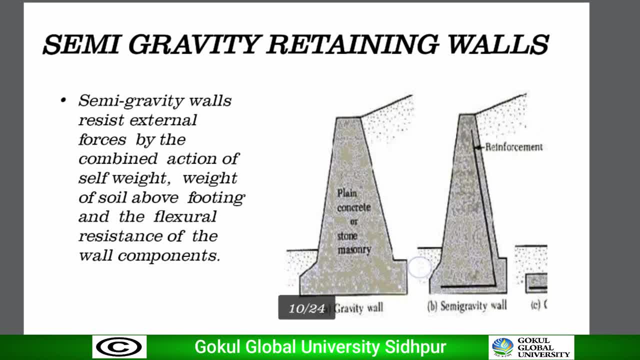 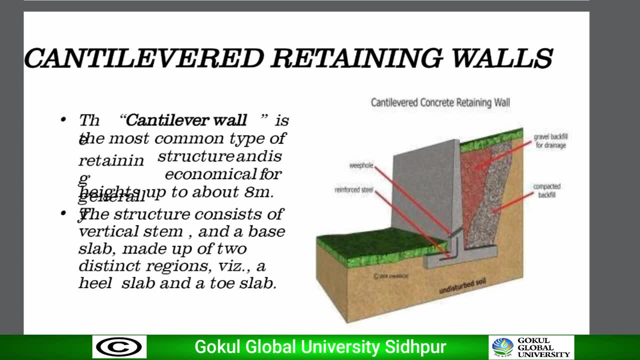 forces in the semi gravity retaining wall and additional reinforcement are provided. third one is cantilever retaining wall, the this is the most common type of retaining wall. it consists of vertical wall called a stem, heel slab and toe slab, which act as a cantilever beam. 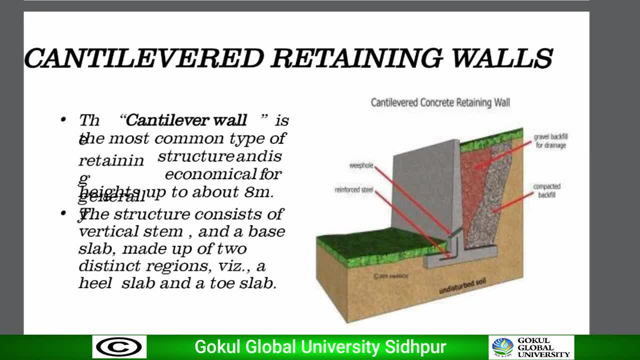 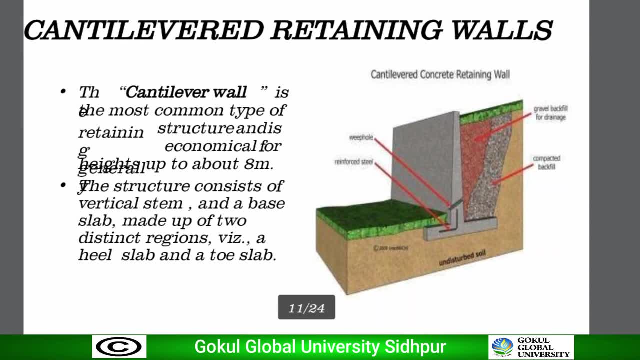 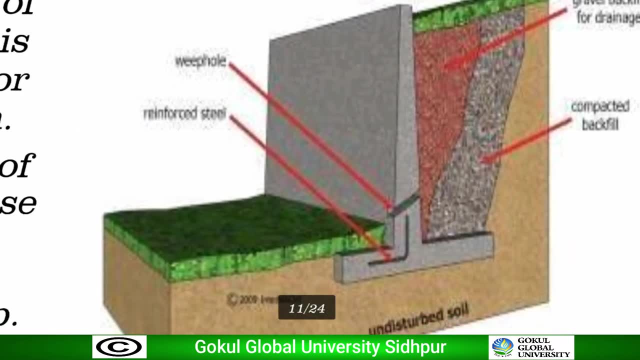 its stability is maintained by the weight of the retaining wall and the weight of the earth on the heel slab of the retaining wall. it is generally used when the height of the wall is six meter. in figure, we can see that different types of the reinforcement still are provided area. 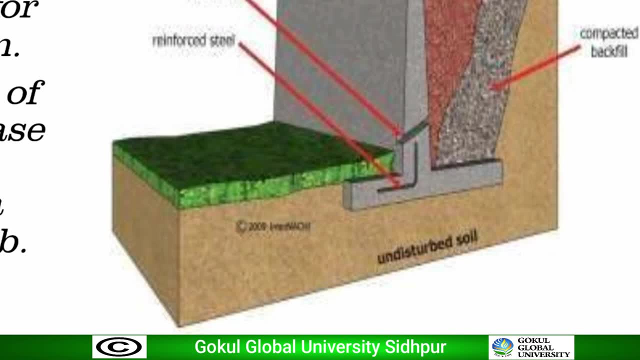 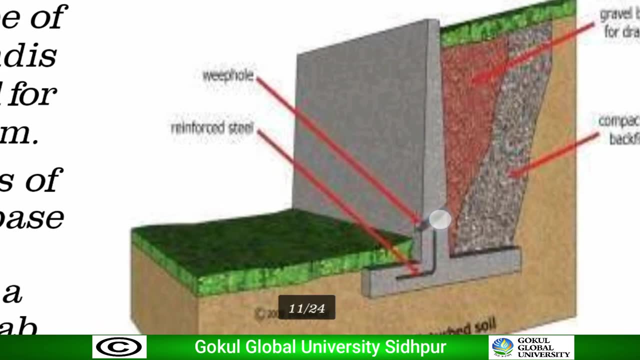 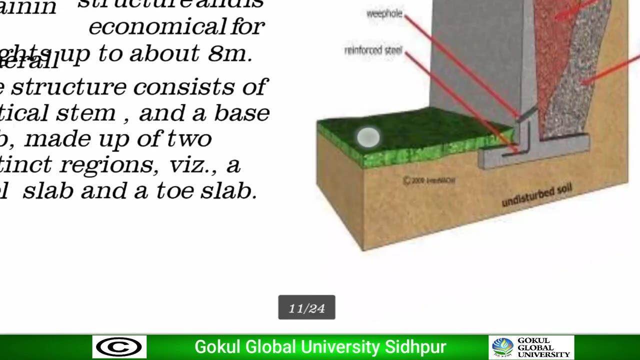 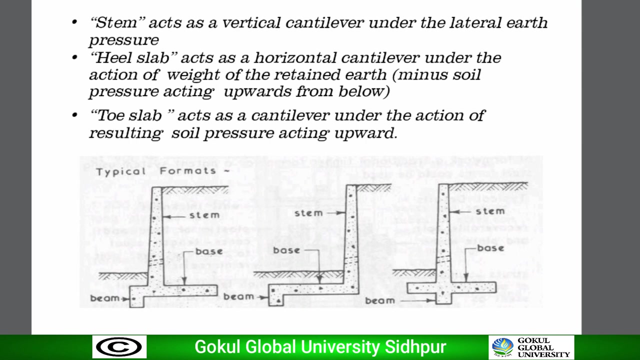 these are the uh below these. below there are undistributed soil and there are upper the backfill. backfill are provided in in cantilever retaining wall there are weep. holes are provided to drain out water during rainy season. cantilever retaining wall resists the horizontal earth pressure as well as other vertical pressure. 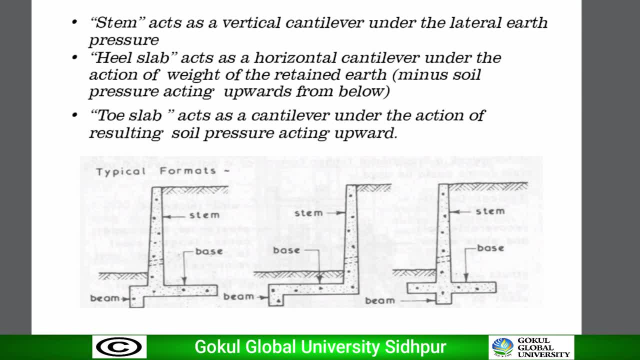 by the way of bending of various components acting as a cantilever. so stem act as a vertical cantilever under the lateral earth pressure. heel slab. act as a horizontal cantilever under the action of weight of the retained earth. toe slab. act as a cantilever under the action of resulting soil pressure acting upward. 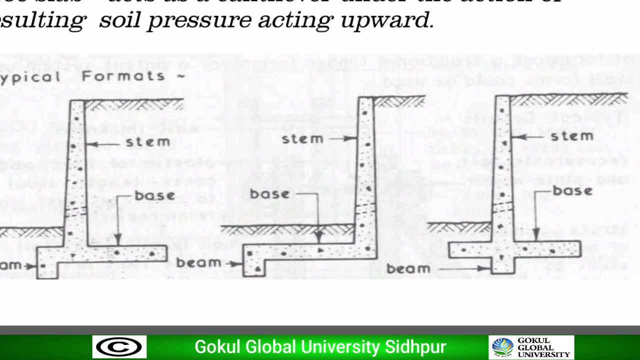 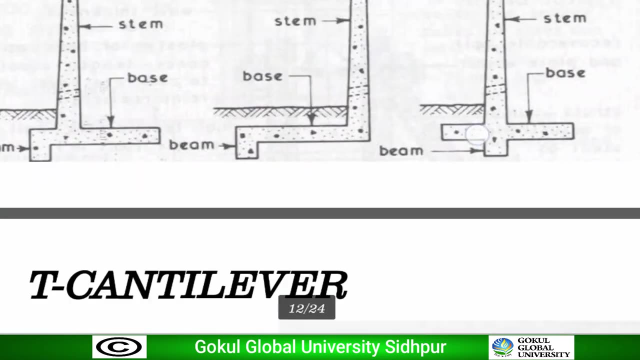 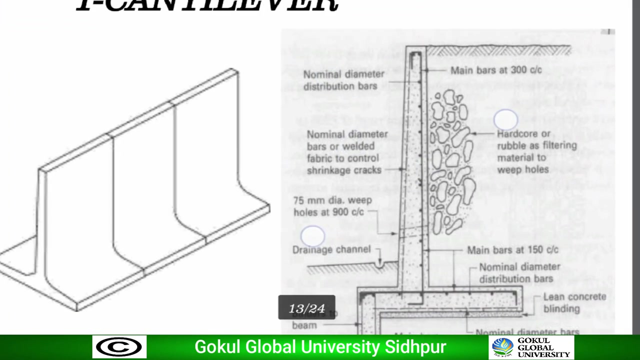 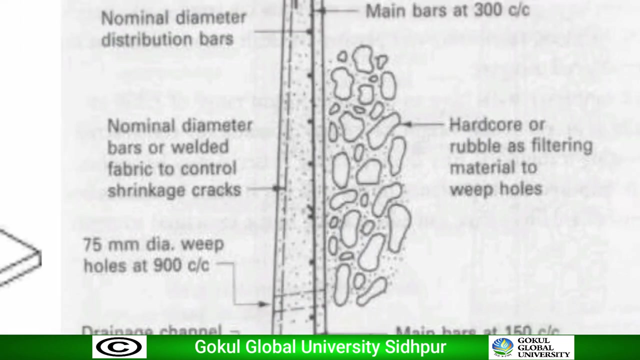 and we can typical format. we can see that cantilever retaining wall are three types: T shape, L shape and T shape with shear cream clear. first one, T cantilever. these are the hand cold or rubber as filtering material to weep holes, generally rubber material. 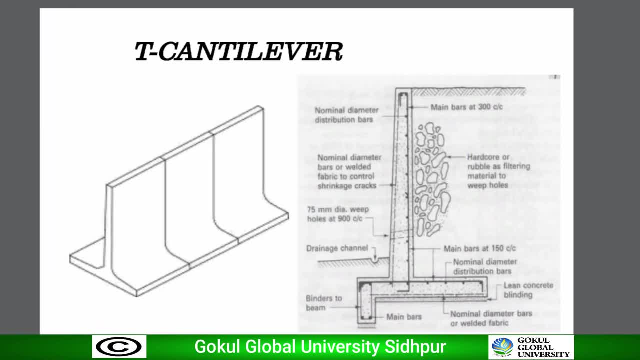 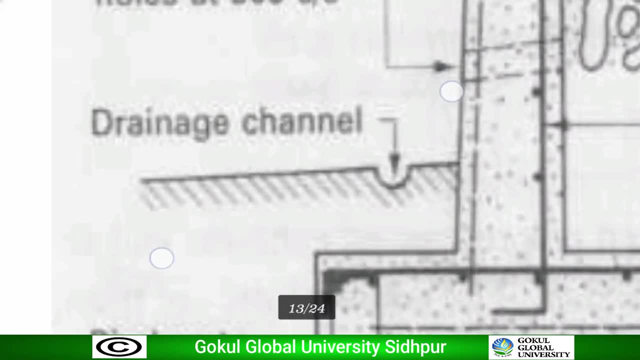 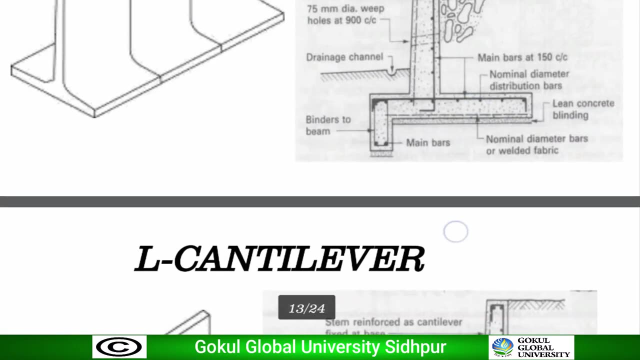 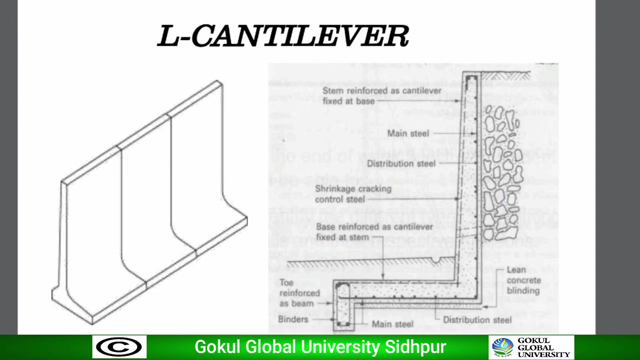 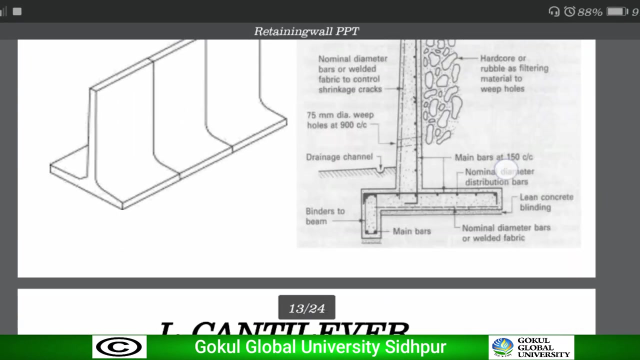 are used to drain out easily water. main reinforcements are provided and these are the drainage channel to drain out the water during rainy season. second one is L cantilever shape. the only difference between T cantilever and L cantilever is only shape, otherwise the draining, otherwise the draining channel, or reinforcement or other rubber material. 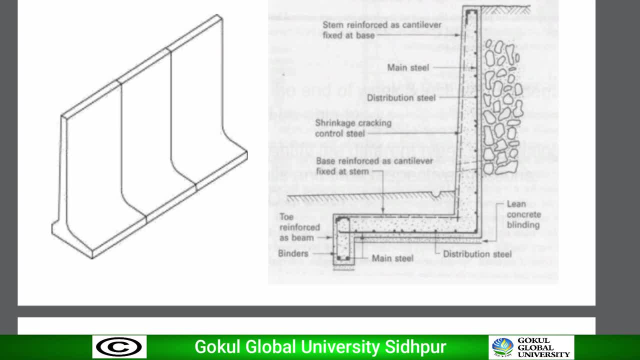 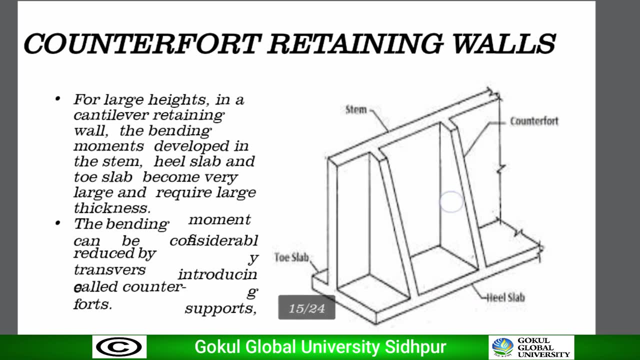 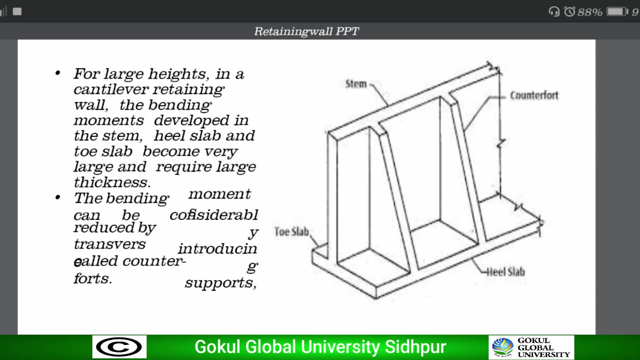 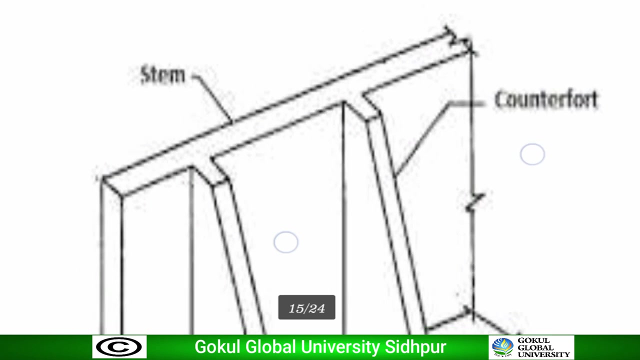 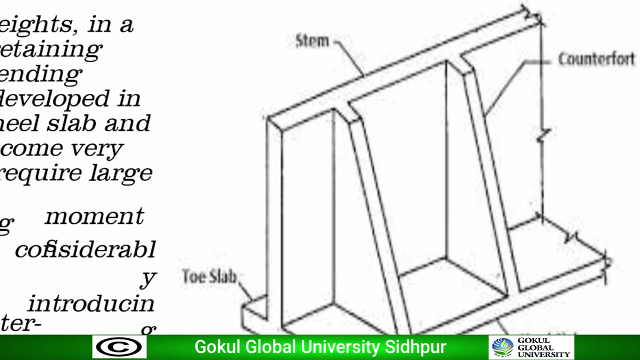 to weep or drain out water is same. the only difference is its shape. okay, now we are discussing counter for retaining wall counter. in the counter for retaining wall, the stem and the base slab are tied together, tied together by counter force at suitable interval. these are the counter force. okay, we can see in the figure. because of provision of counter for the vertical stem is tied together at a suitable interval. these are the counter force. okay, we can see in the figure. because of provision of counter for the vertical stem is tied together at a suitable interval. these are the counter force. okay, we can see in the figure. because of provision of counter for the vertical stem is tied together at a suitable interval. these are the counter force. okay, we can see in the figure. because of provision of counter for the vertical stem is tied together at a suitable interval. these are the counter force. okay, we can see in the figure. because of provision of counter for the vertical stem is tied together at a suitable interval. these are the counter force. okay, we can see in the figure. because of provision of counter for the vertical stem is tied together at a suitable interval. these are the counter force. okay, we can see in the figure because of provision of counter for the vertical stem. 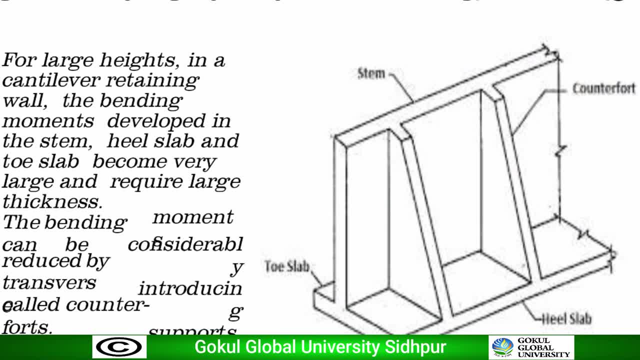 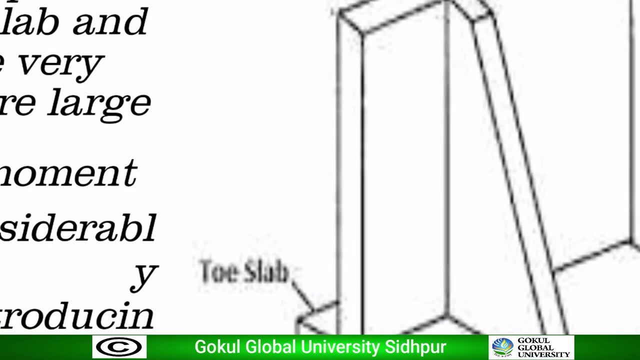 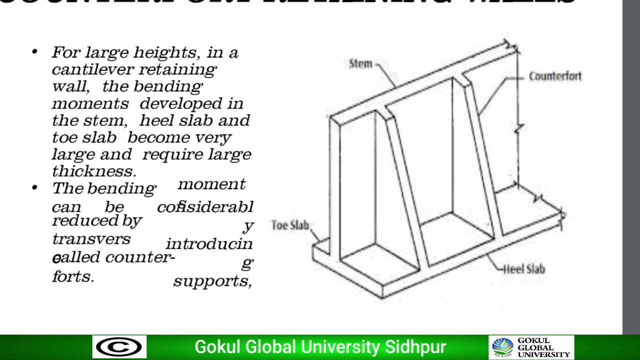 as well as the heel slap, act as a continuous slap, in contrast to the cantilever of cantilever retaining wall. the toe slap, however, act as a cantilever bending upward. this toe slap act as a cantilever bending upward. the counter foot: the counter foot retaining wall, the in the counter foot retaining. 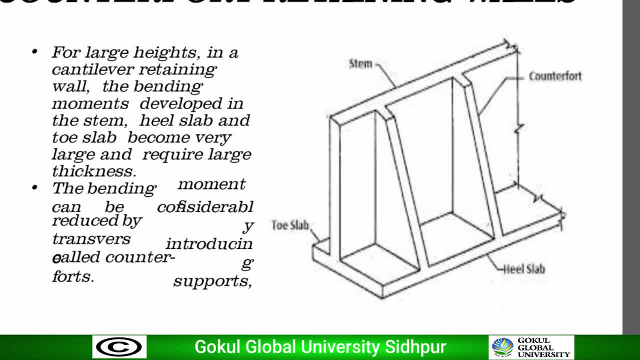 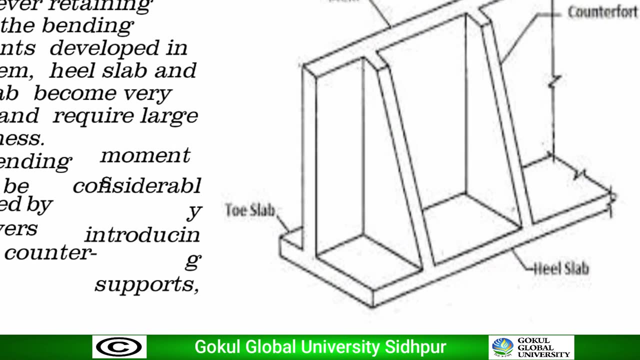 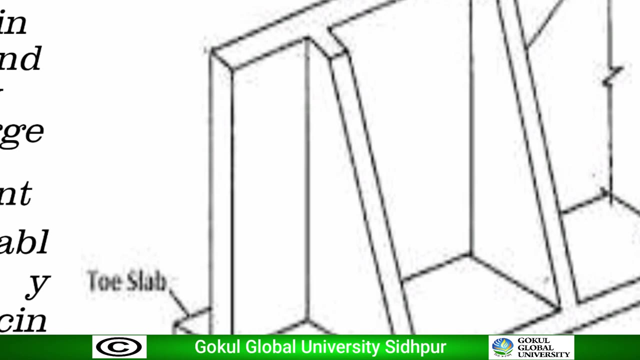 wall. the counter foot act as a tension member to support the stem and reduce bending moment in it. it is also provided support to heel slap. it is also provided to support heel slap and reduce bending moment in it. generally the counter foot are spaced at approximately one-third height of the wall. the 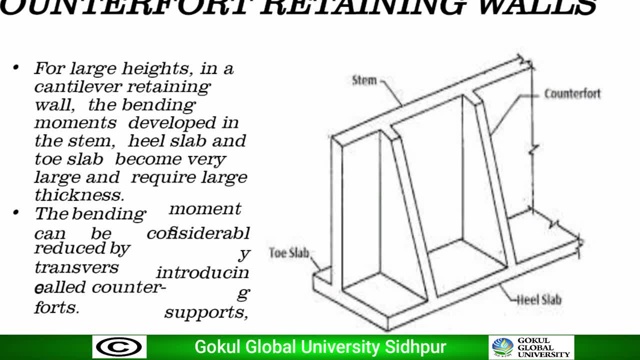 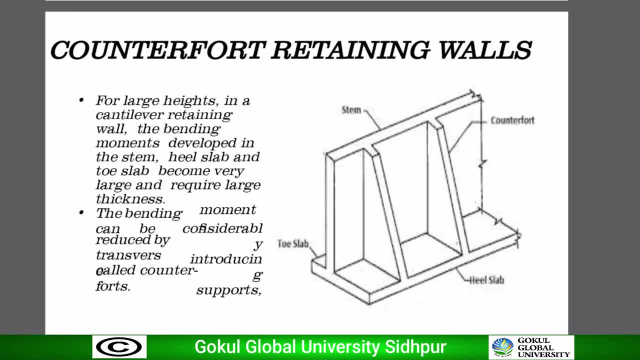 stability of the retaining wall is maintained by the weight of the earth and the pressure of the wall is maintained by the weight of the earth on the base lap. on the base lap and its self weight counter foot retaining wall are economically for height over about six meter when there is a requirement of 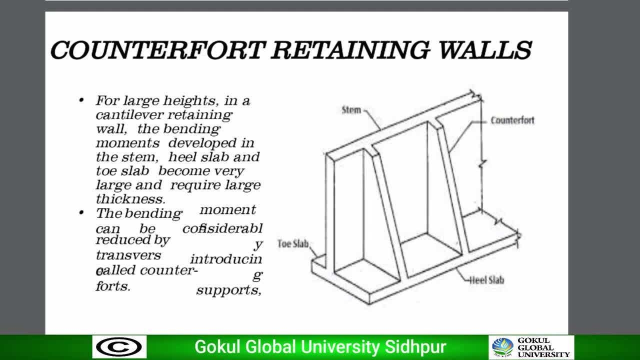 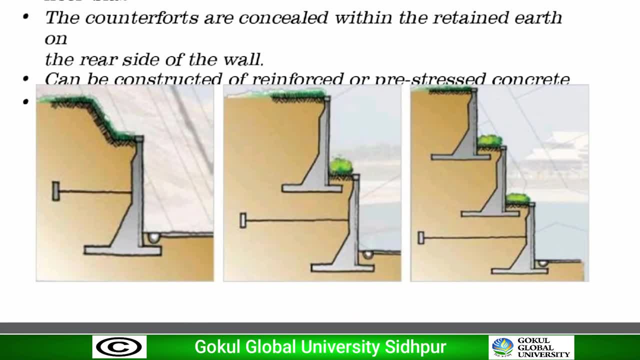 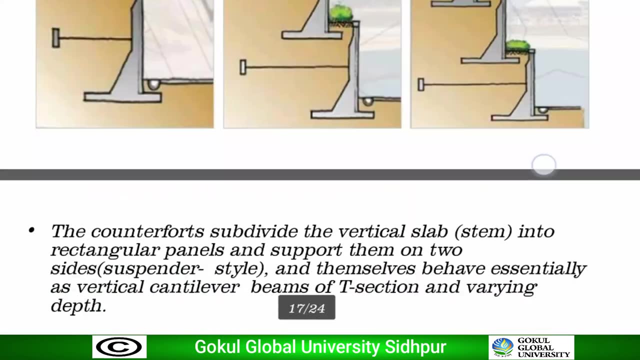 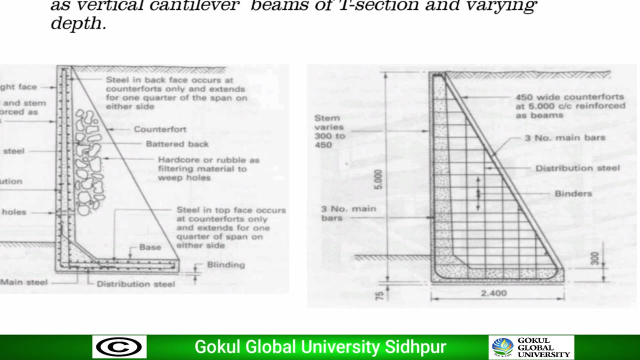 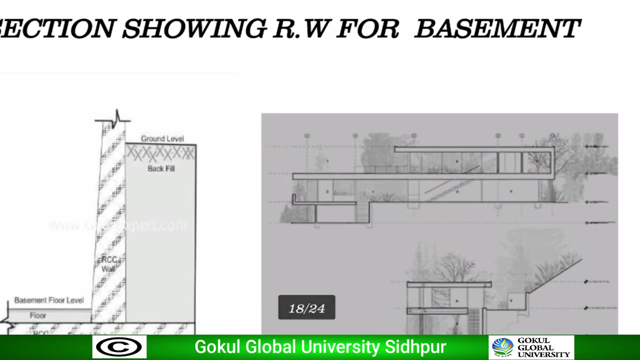 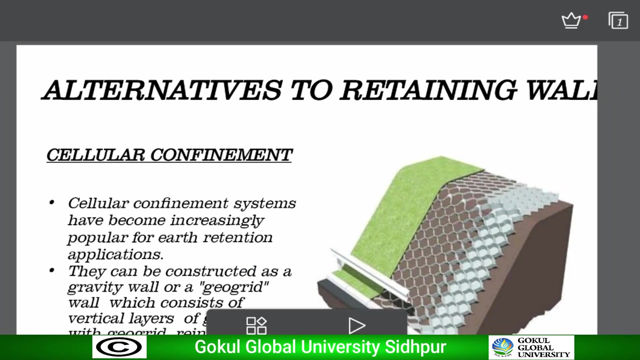 height above six meter counter foot retaining wall are used. okay, these are the. in the figure you can see that the counter foot retaining wall are constructed at different side. these are the Human nic bene deep matting Toe perform function in the i's assgets to the base lap and these are the counter. user reinforcement i provided in counter for retaining wall and these are the section show of retaining wall counter for retaining wall. these are the sections. own retaining wall is removing bl일�ling in the base lap. 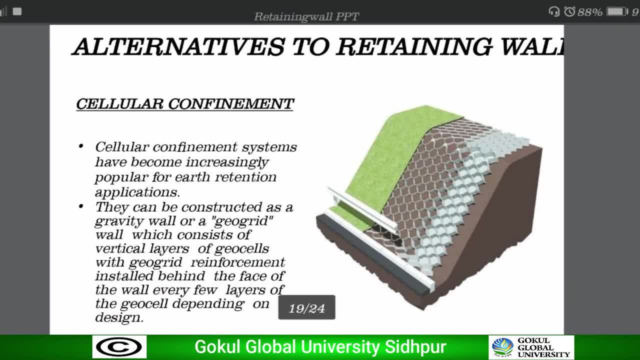 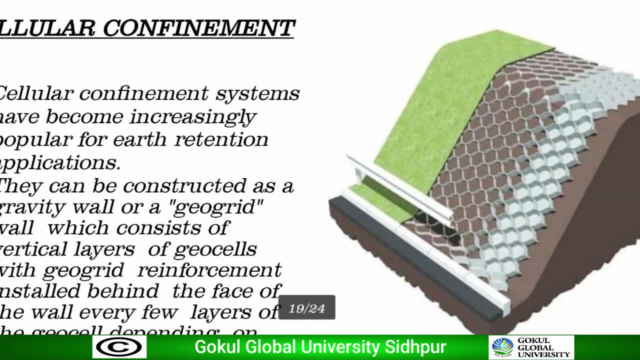 in alternative to retaining wall. alternative to retaining wall means the material is alternate by the different types of new material like geocell, geonet, geo confinement. the first one is cellular confinement. cellular confinement system have become increasingly popular for the earth retention application. nowadays geonet geomembrane is easily available in the market and it is 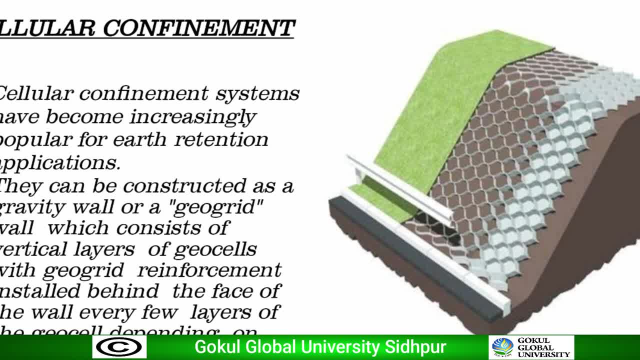 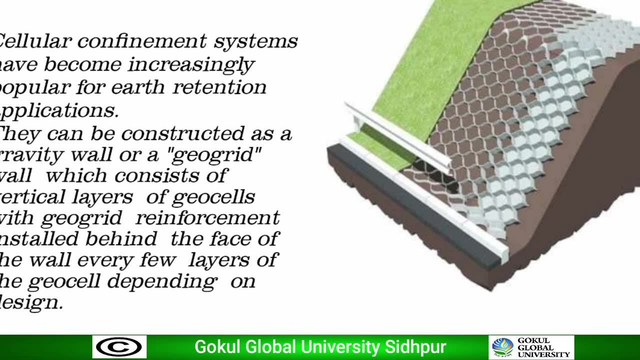 cellular confinement means its bonding strength is good and it is easily economically. economically so they are constructed as a gravity wall or as a geo grid wall, which consists of vertical layer of geocell with geogrid enforcement installed behind the face of the wall, every few layer of the geocel, depending on design. in the figure we can see geocell week. 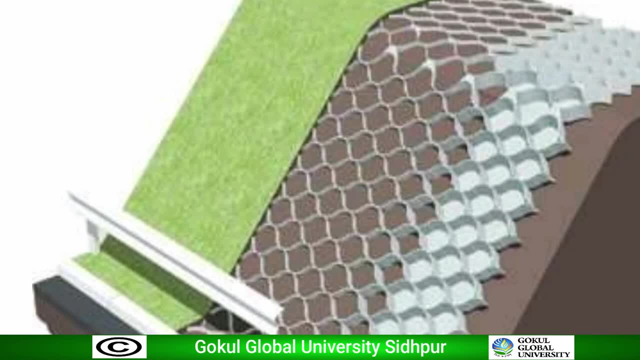 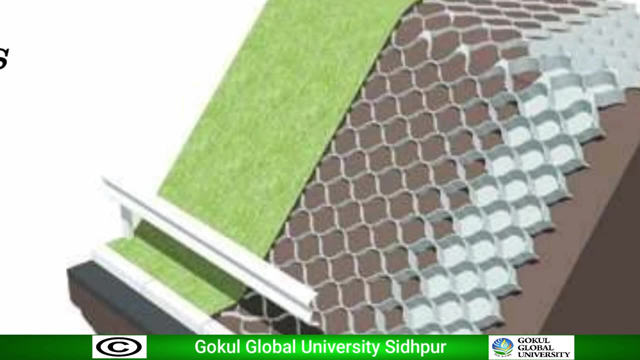 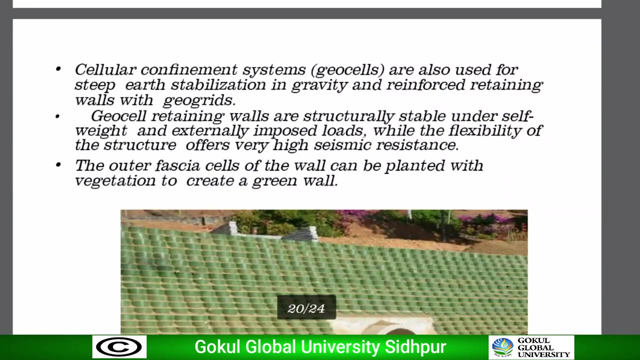 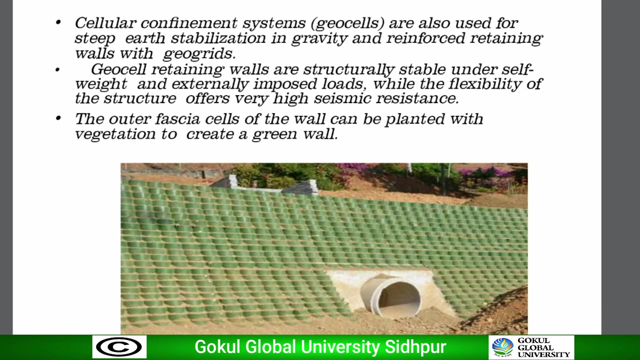 in the in the figure we can see, geocell are provided and the reinforcement and after that reinforcement are provided and binding with this. geocell confinement. cellular confinement system or geocell are used for the steep earth stabilization in gravity and retaining wall with geo grid, geocell, geo grid, geo. 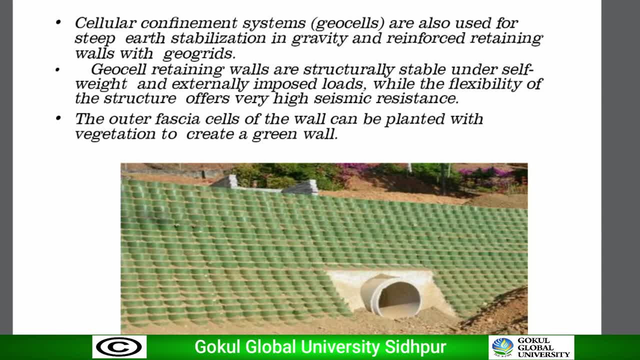 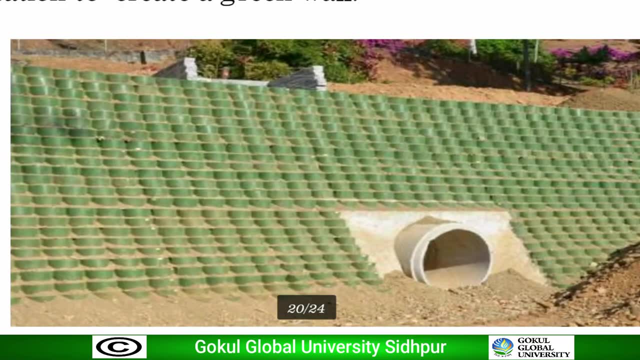 net. these are the reinforcement material nowadays easily available in the market and used widely in retaining wall design. the outer phases cell of the wall can plan it with vegetation to create a green wall. in figure we can say that green valley green wall is provided this one is one type of cellular confinement. 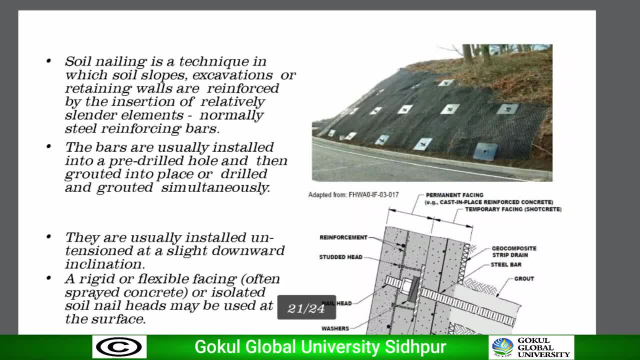 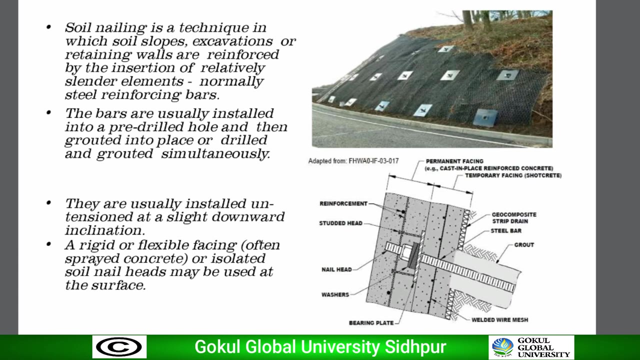 okay. nowadays, soil test, soil nailing- is a technique which soil slope excavation or retaining wall are reinforcement by the insertion of relatively slender element, normally steel reinforcement bar. they are usually installed in pretension pre-drilled hole and then grouted with concrete and a rigid or flexible facing or isolated soil nail heads may be used. 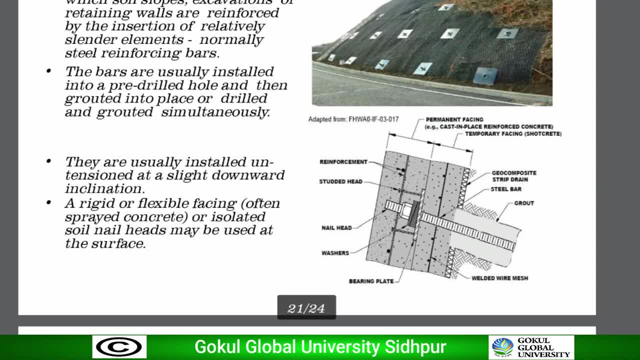 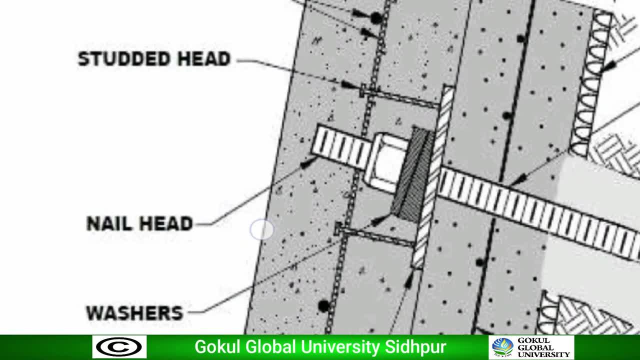 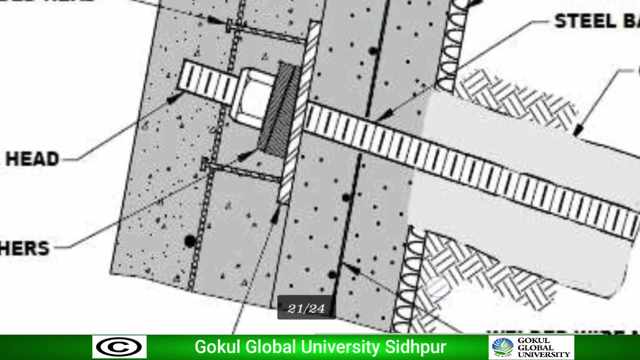 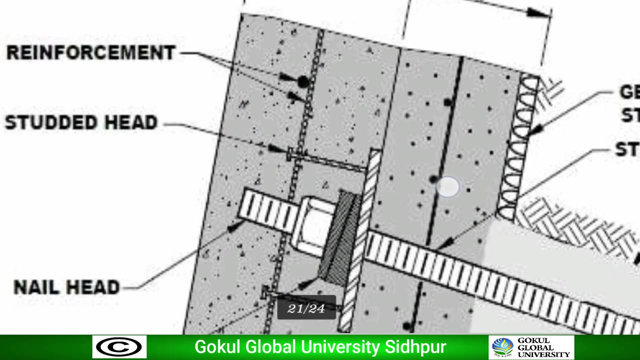 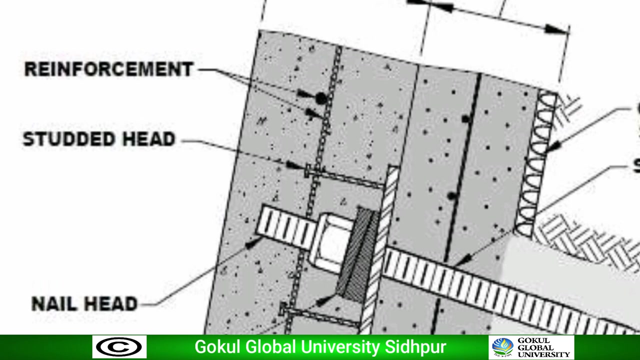 at the surface to retain the slope material or to slope material. these are the swelling soil nailing. this is soil nail head. these are the washers the bearing plate are provided. these are the welded wire mesh and these are the steel bar. we can see that in the figure and this one is reinforcement are provided on the outer side of reinforcement are provided on the outer side of nail head. 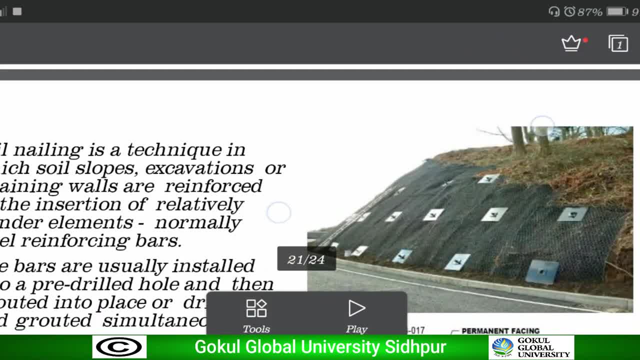 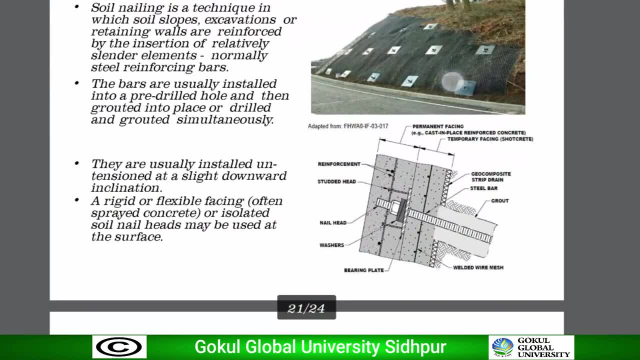 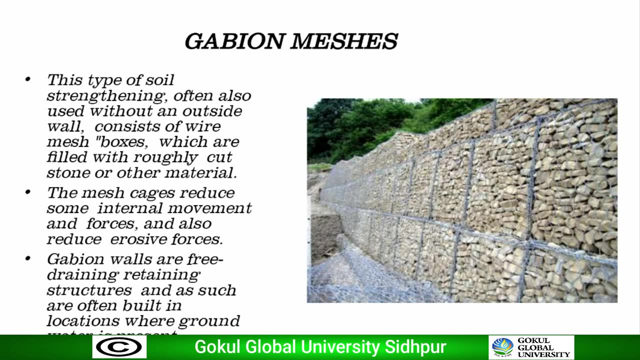 and this figure show side figure means the where there are the soil nailing our done gave your message on. well, we can see that one and I'm LG highway- I think I'm the Inam downward Gabion message- are provided these types of soils, tentin Ofan, also used with out and out problems and we can. 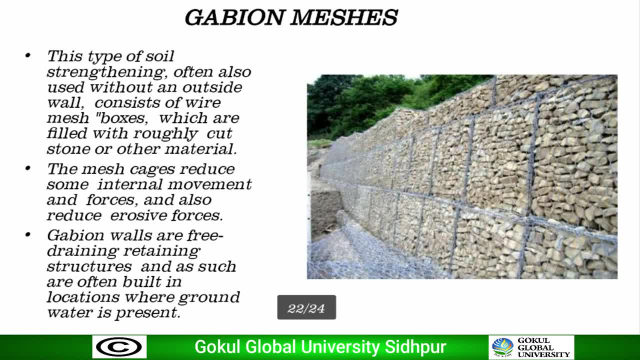 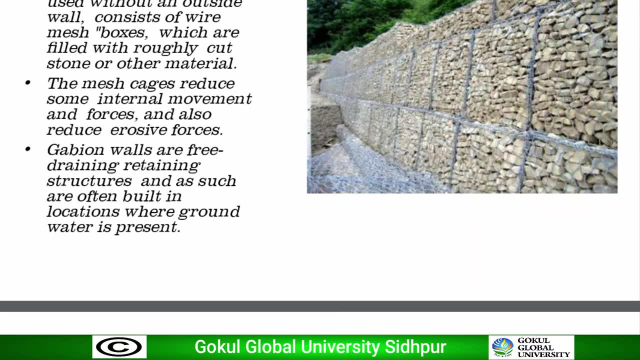 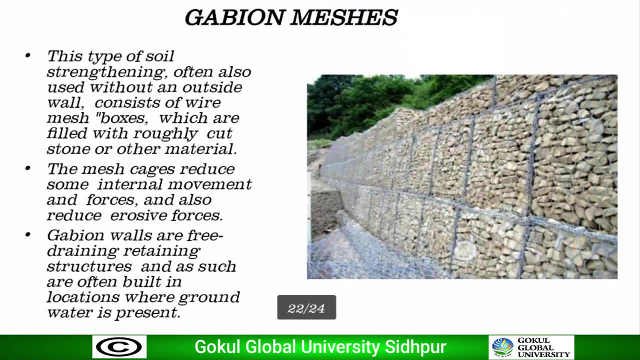 An outside wall consists of wire meshes boxes which are filled with roughly cut stone or other material. Gabion wall are free draining retaining structure and such are often built in location where ground water is present, Means if there is a ground water present, we can construct a gabion meshes. 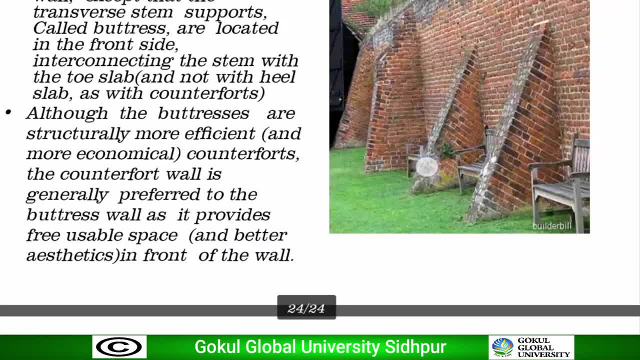 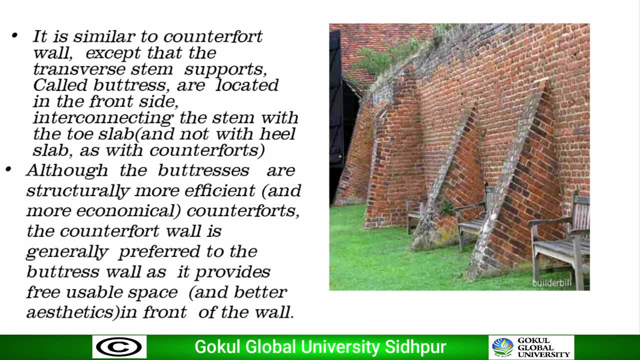 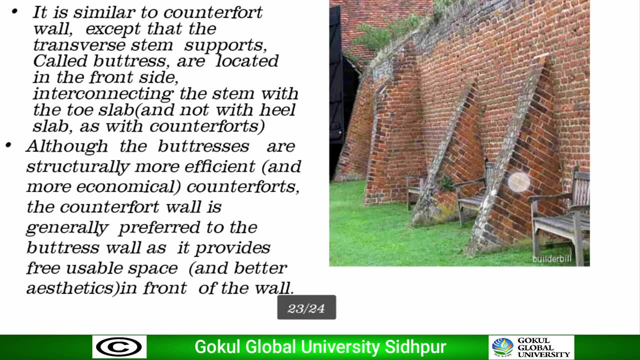 And last one is buttress wall. Buttress wall- it is similar to counter fort- expect that the transverse stem support, called it buttress, are located in front side, interconnecting the stem with the toe slab, And all through buttress wall is provided a free, usable space nowadays ok. 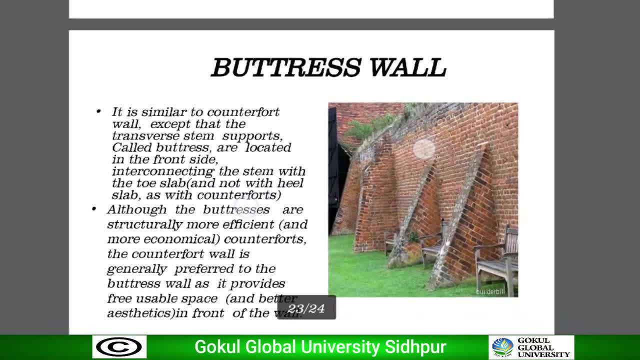 So these are the different types of retaining wall we are discuss in this presentation. Thank you, Thank you, Thank you.